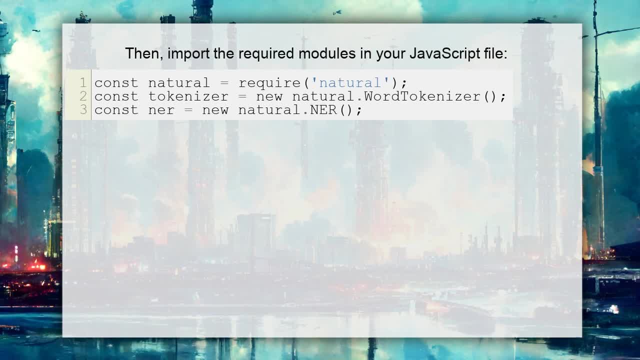 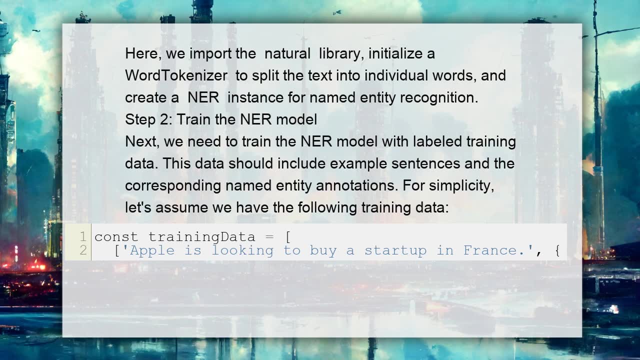 Then import the required modules in your JavaScript file. Here we import the Natural Library, initialize a word tokenizer to split the text into individual words and create an NER instance for Named Entity Recognition. Step 2. Train the NER model next. 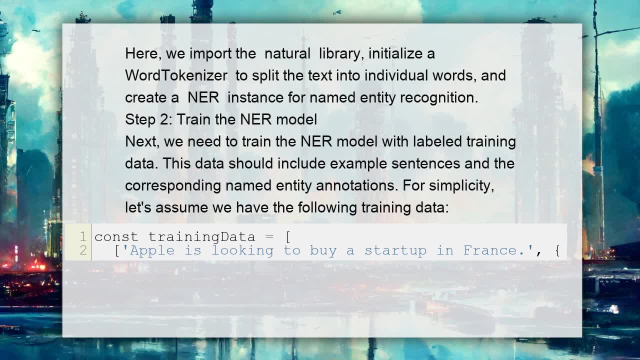 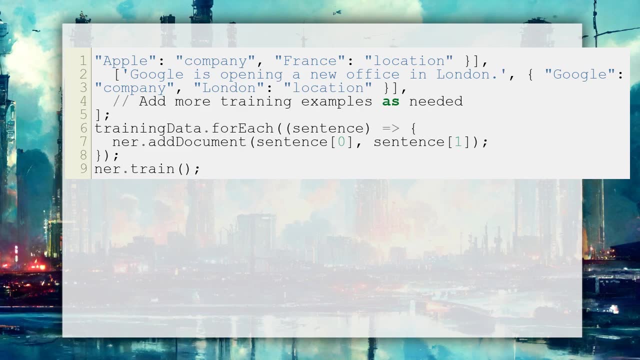 We need to train the NER model with labeled training data. This data should include example sentences and the corresponding Named Entity Annotations. For simplicity, let's assume we have the following training data And here is the result. Let's continue In this example. we provide two sentences and their corresponding Named Entity Annotations. 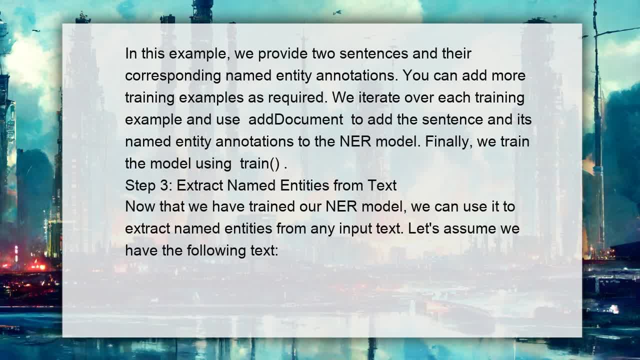 You can add more training examples as required. We iterate over each training example and use add document to add the sentence and its Named Entity Annotations to the NER model. Finally, we train the model using train Step 3.. Extract Named Entities from text now that we have trained our NER model. 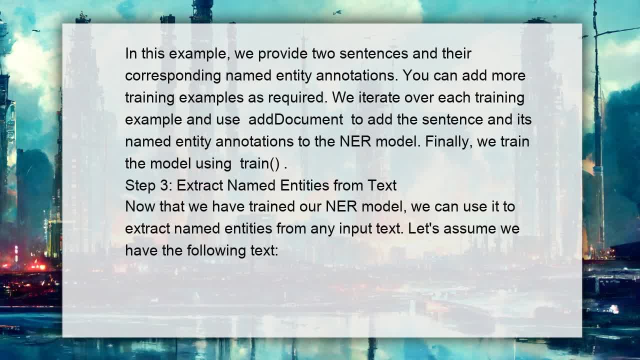 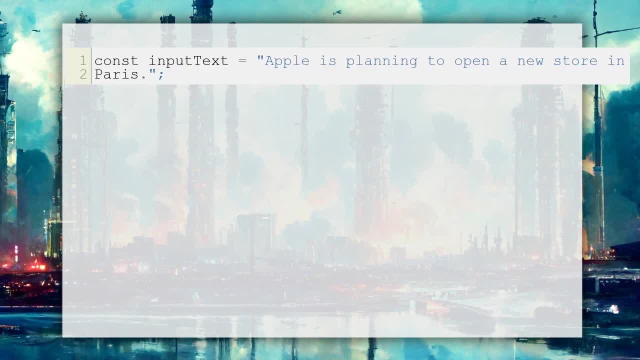 Step 4.. We can use the NER model to train the model. We can use it to extract Named Entities from any input text. Let's assume we have the following text: And here is the rest of the code. Let's continue. 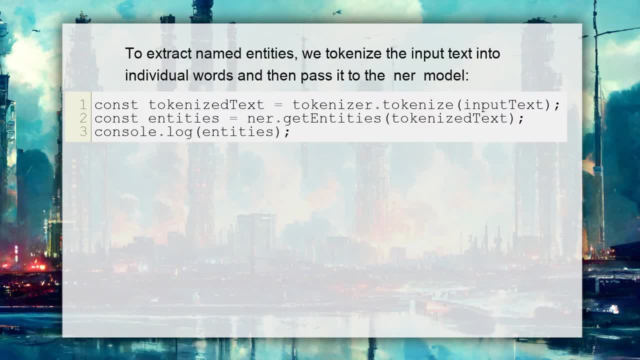 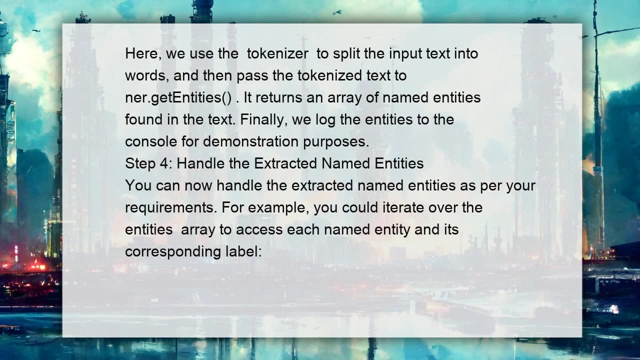 To extract Named Entities. we tokenize the input text into individual words and then pass it to the NER model. Here we use the tokenizer to split the input text into words and then pass the tokenized text to NER: Get Entities. 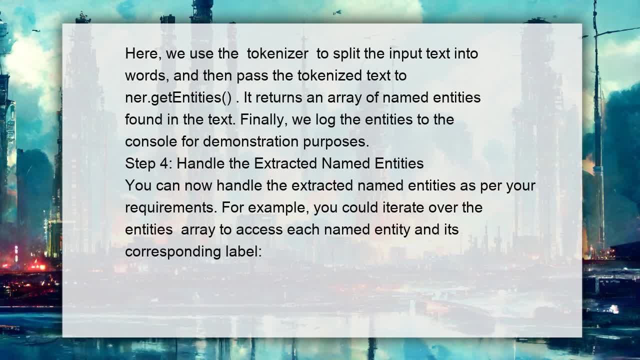 It returns an array of Named Entities found in the text. Finally, we log the entities to the console for demonstration purposes. Step 4. Handle the extracted Named Entities. You can now handle the extracted Named Entities as per your requirements. For example, you could iterate over the entities array to access each Named Entity. 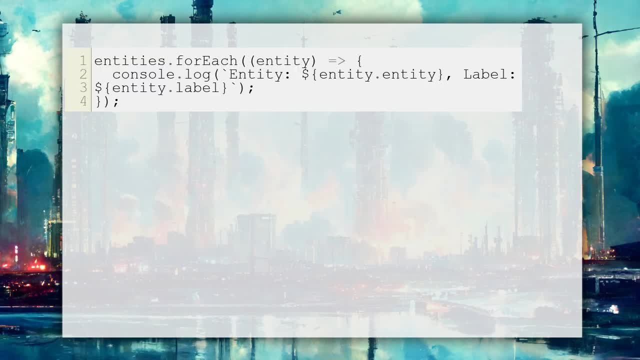 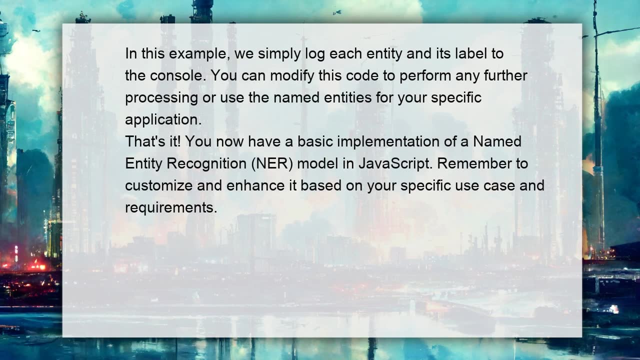 and its corresponding label. And here is the rest of the code. Let's continue In this example. we simply log each entity and its label to the console. You can modify this code To perform any further processing or use the Named Entities for your specific application.